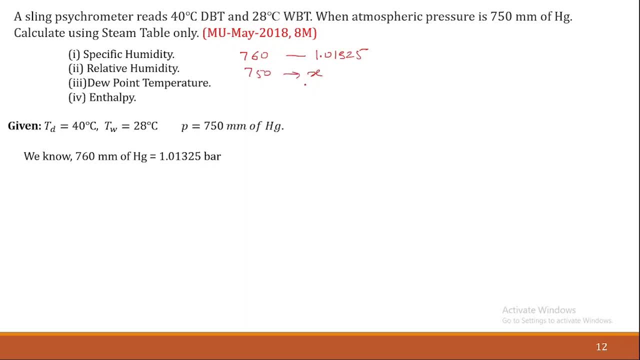 it is. So if I solve for x, I will get answer like this, Which is equal to. here instead of x we have P equal to 750 by 760 into 1.01325.. So if I solve this one, I will get answer for the atmospheric pressure in bar as 0.99992 bar. Now let's find. 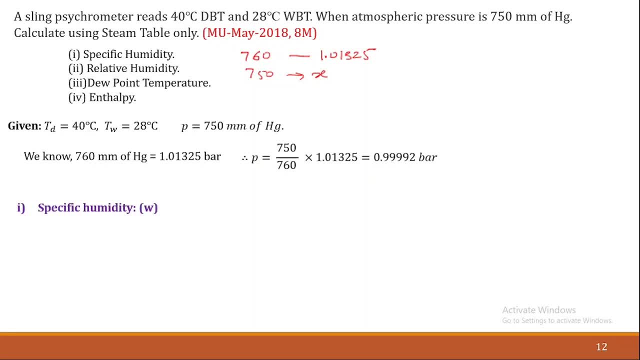 specific humidity. What is specific humidity? It is nothing but the mass of water vapor present in air per kg of dry air. So we get that specific humidity using this formula, which is equal to 0.622, into Pb upon P minus Pb. Anyways, this Pb is: 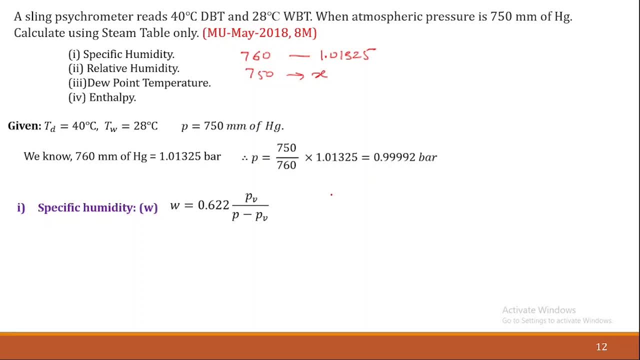 nothing but partial pressure of water vapor present in the air, and P is barometric pressure or atmospheric pressure. So to find out this specific humidity, first of all we should know Pb, because P is already known to us. So to find out this Pb, we have carrier equation. 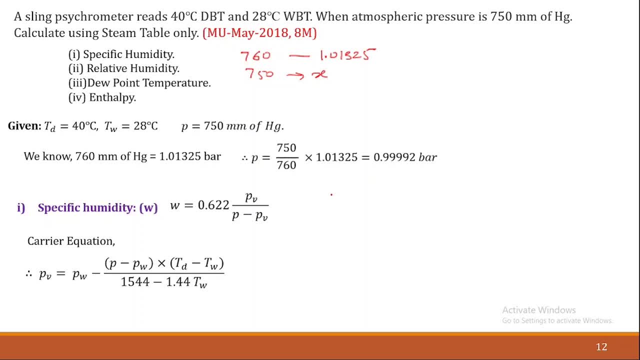 which is equal to Pb, equal to Pw minus P minus Pw into Td minus Tw, upon 1544 minus 1.44 Tw. In this formula, Pw is nothing but the saturation pressure of the air. So this Pb is nothing but the radiative pressure corresponding to wet well temperature. So that can be written. 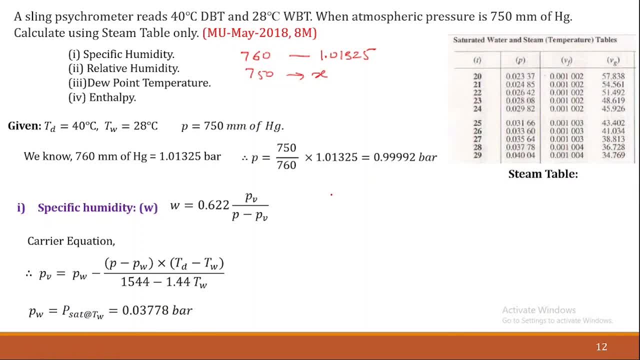 as like this. So Pw is nothing but the saturation pressure corresponding to wet well temperature. So in our problem wet well temperature is given as 28 degree C. So from the steam table, if I find out the temperature scale, that is saturated water and steam, that is from the 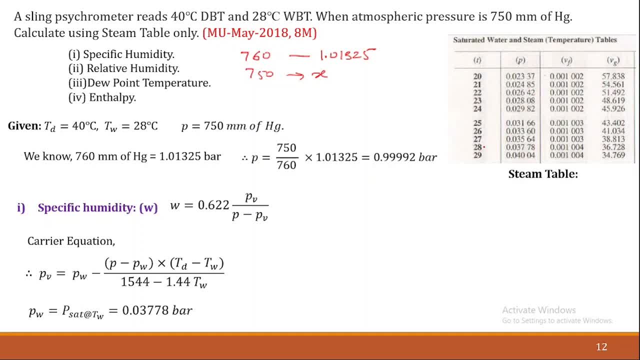 steam table, the temperature table, we get the saturation pressure corresponding to 28 degree celsius. so this is equal to 0.03778 bar. if i write this equation, i will get here now. if i put this value in this formula, i will get the value of partial pressure of water vapor like this: 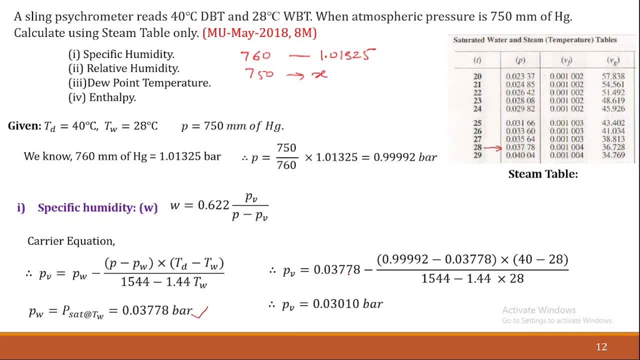 0.03778. that is the pw. then we have atmospheric pressure 0.99992 minus 0.03778, multiplication the drywall temperature 40 degree celsius and wetwell temperature 28 degree celsius, and in the numerator denominator we have 1544 minus 1.44 into wetwell temperature 28. 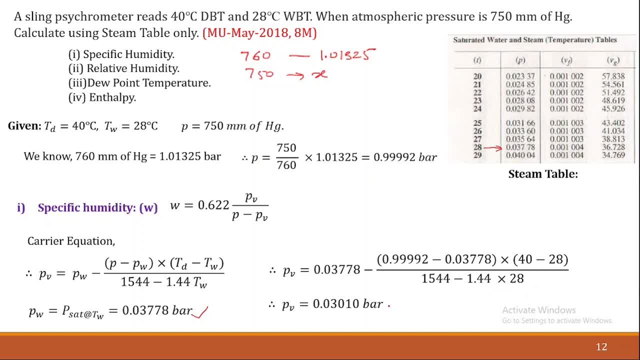 degree celsius. so if i solve this, i will get answer for partial pressure of water vapor as 0.03010. now, if i put this value in this relation, i get answer as 0.1- 0.0193 kg per kg of dry air. okay, 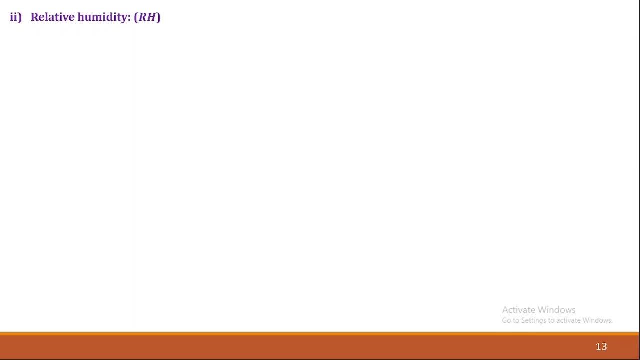 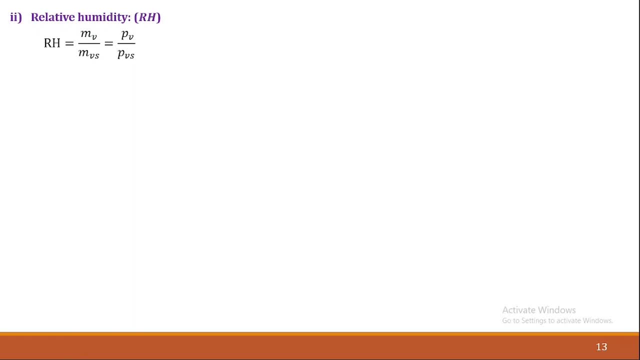 so if i write this, i will get mass of water vapor upon mass of water vapor at saturated conditions, so mv upon mps. now if i solve for mu upon mps, i get that relative humidity also equal to pv upon pvs. that is partial pressure of water vapor divided by partial pressure of. 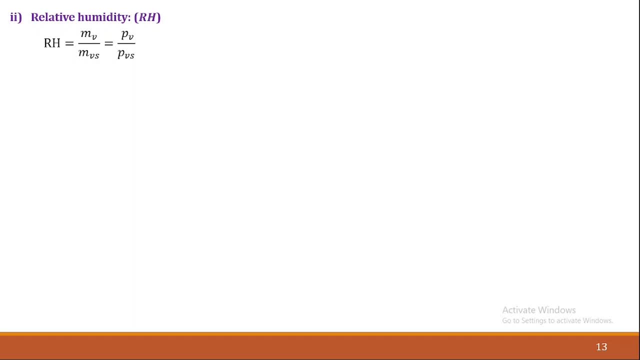 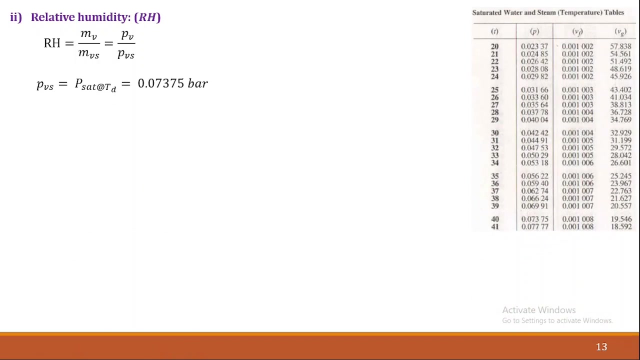 water vapor at saturated condition. okay, now we, in this formula, we have already find, found out pv, now let us find out pvs. so what it is? it is nothing but the saturated pressure corresponding to drywall temperature. so pvs is nothing but saturated pressure corresponding to drywall temperature. 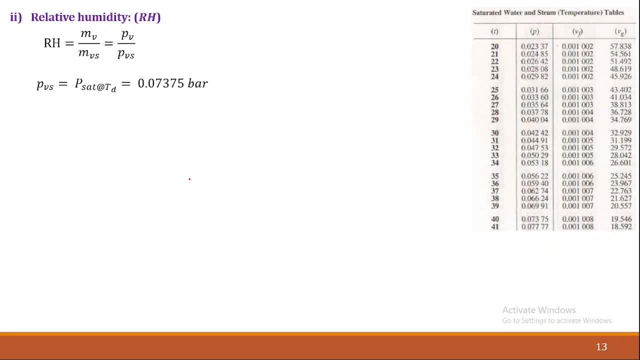 so in this problem the drywall temperature is 40 degree celsius. so from the steam table corresponding to 40 degree celsius drywall temperature we find saturated pressure which is nothing but pvs point zero, seven, three, seven, five bar. now, if i put the value of this in rs, 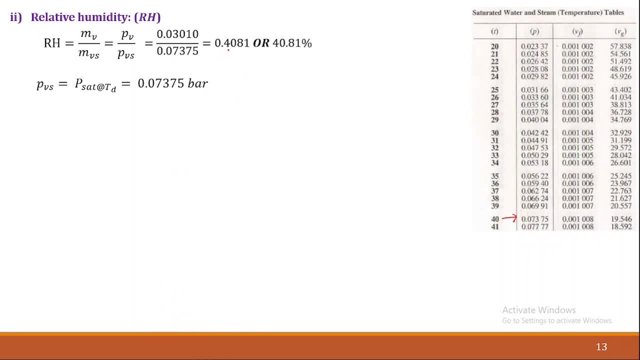 relation, i'll get the value of rs as point four zero eight, one which is also equal to written as 40.81 percent. this is relative humidity. now let us find out dew point temperature. what exactly is dew point temperature? it is nothing but the saturation temperature corresponding to partial pressure of. 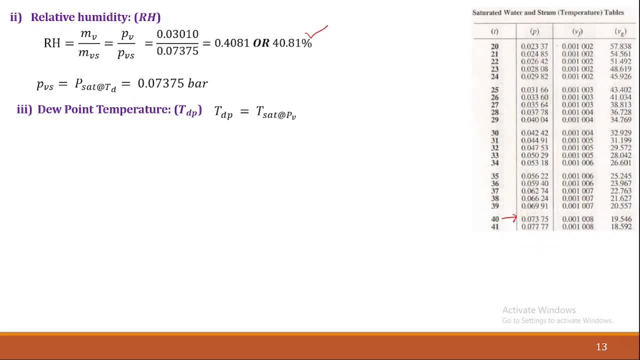 water, water vapor, right. so partial pressure of water vapor is known to us. it is equal to 0.03010. so from the steam table, again using the pressure table, if i plot or if i get the value corresponding to 0.0301, i get the saturation temperature as 24.10 degree celsius. so 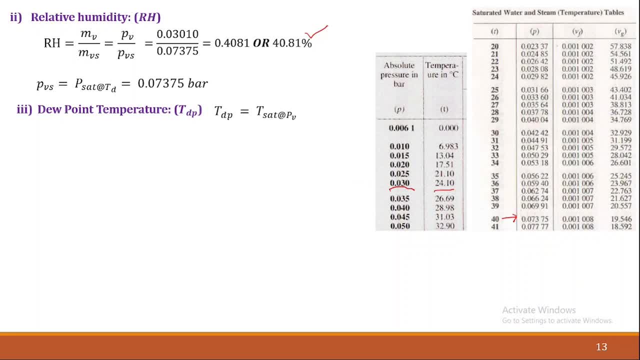 corresponding to this pressure. from the steam table we can get the value of dew point temperature as 24.10 degree celsius. the meaning is that the air given in the problem will condense at 24.10 degree celsius when the temperature is reducing without changing the partial pressure of. 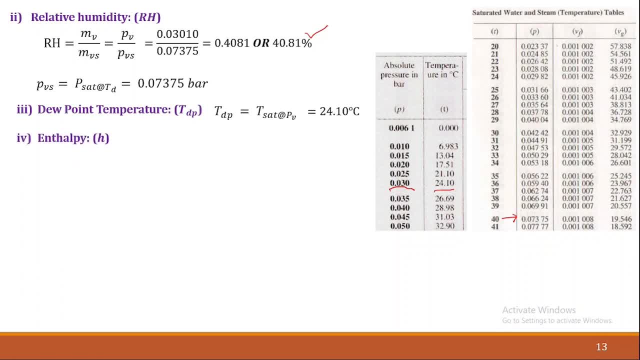 water. now next is enthalpy. so the formula to find out the enthalpy of the moisture is equal to 1.005 td plus w into 2500 plus 1.88 into td. so moist air enthalpy is equal to 1.005 into td. so td given in the problem is 40 degree celsius right and w we have already. 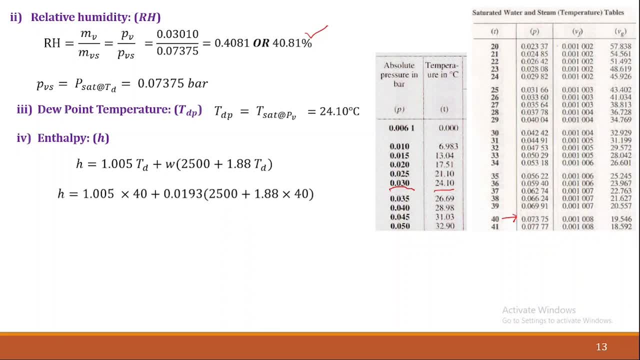 already found out. so if i write for the h value, that is, enthalpy of moist air, then it is equal to 1.005 into 40 degree celsius travel temperature, plus 0.0193 into 2500, plus 1.88 into 40.. 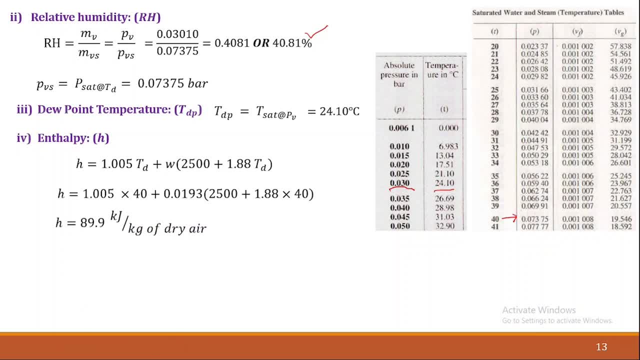 so if i write, if i solve for this, i'll get enthalpy as 80- 89.9 kilojoules per kg of dry air. this way we have solved all the values in the problem. thank you.